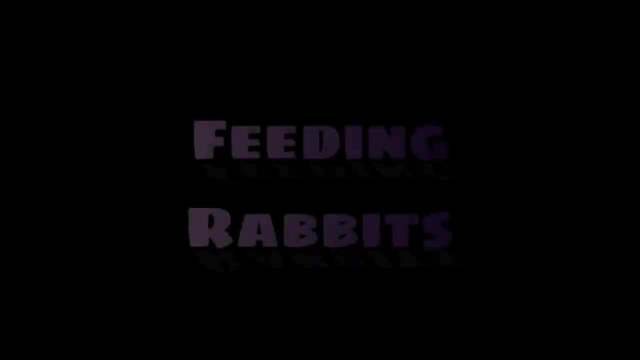 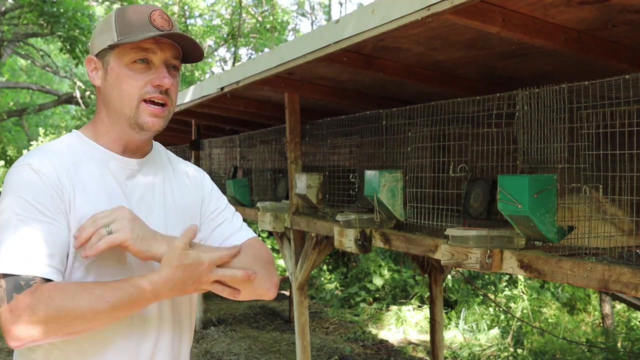 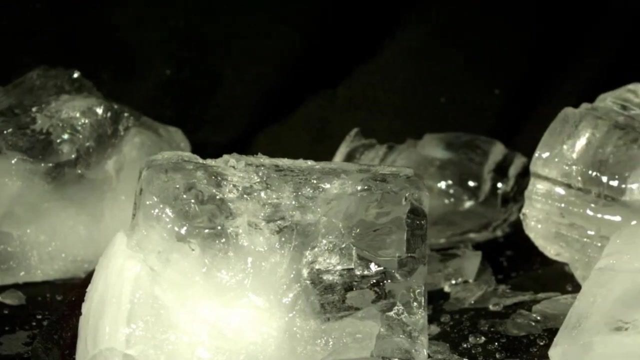 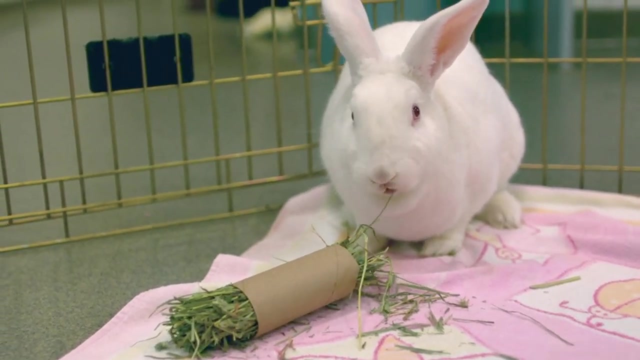 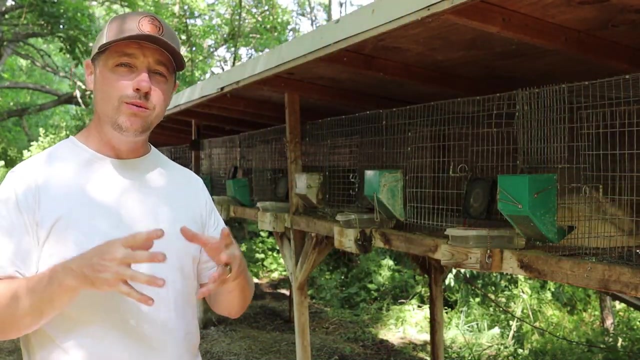 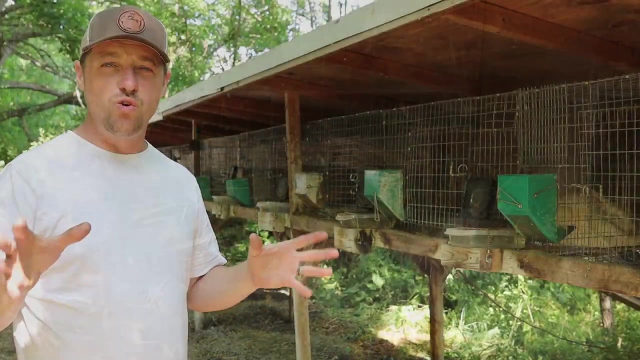 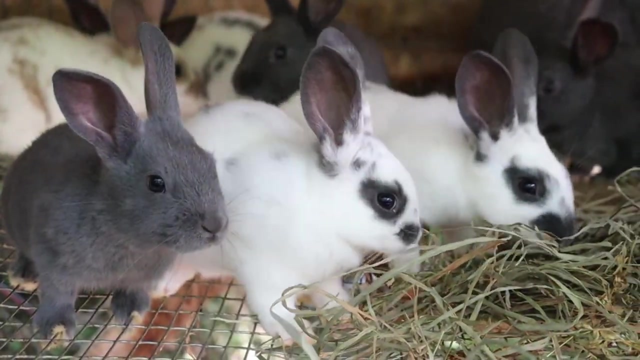 from the heat. But that's not the number one reason. You know there's some things that you can put in a rabbit's cage that would surprise you that they would just completely devour, like a big block of ice or a potato or a corn cob. But you know those things- ice cubes- are very beneficial for your rabbits in the winter time, It's good for their teeth, It's great in the summertime. But as far as like potatoes go or corn cobs, you know I would try to resist the urge to just throw whatever you want, because when it comes to feeding your rabbit, you do want to adopt some sort of a system where you're feeding the same amounts approximately, because rabbits gain weight really easily, especially when you're feeding them with the same amount of food. 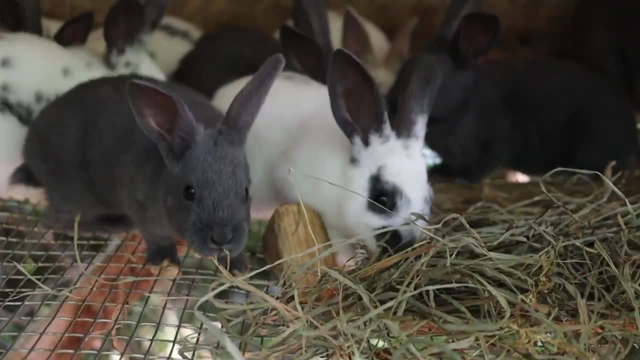 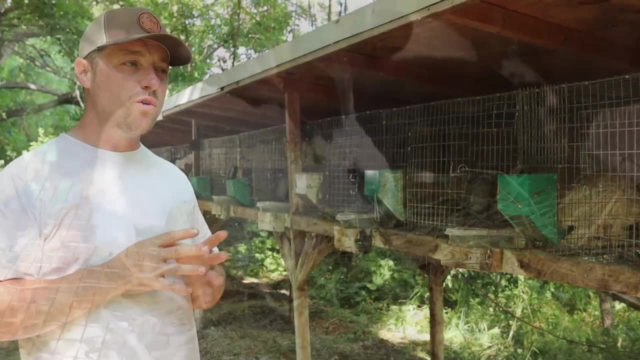 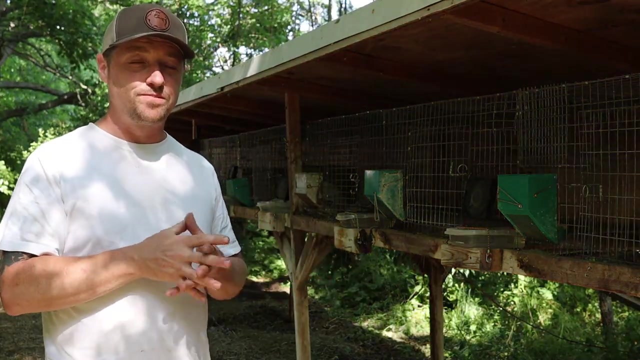 Especially those that don't get as much exercise as other rabbits. And you know that will affect the health of your rabbit. I mean, quickly, It will affect the health of your breeding. So you know, folks often think that because of their diets. you know this is the reason why they're failing. You know, when you're raising your rabbits it's important that they have good nutrition. 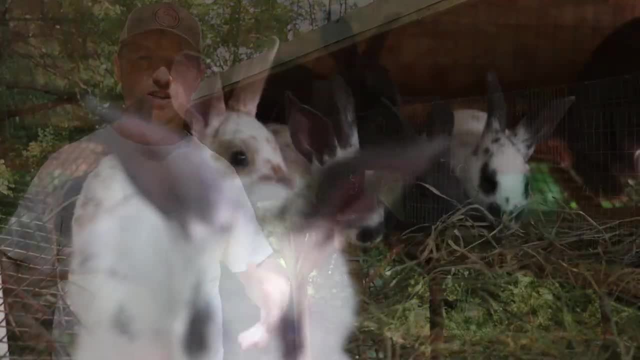 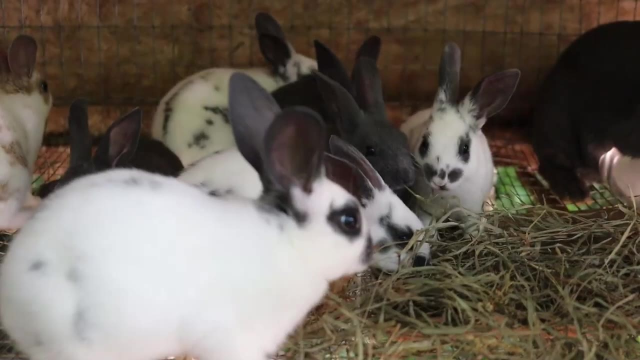 You want. you know, a really common question is: what can I feed my rabbits to make sure they grow faster or they grow out better? And you're really looking for good grow genetics, looking for good nutrition and good feed. you want to stay away from the feed that. 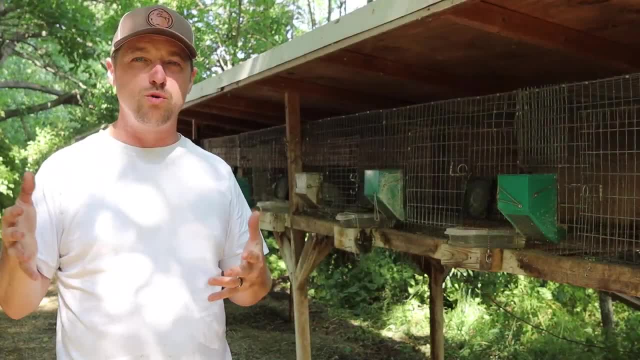 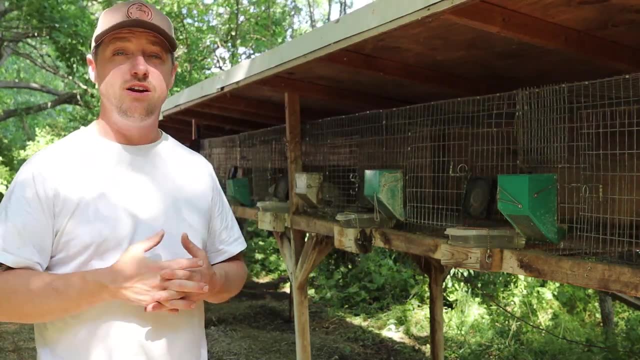 has fruit loops or high sugar or just doesn't meet the fiber or protein needs of a young rabbit, which is right around 16% protein, 17 to 18% fiber. you know, on a low end you always want to provide hay, that's gonna help you, but you know. 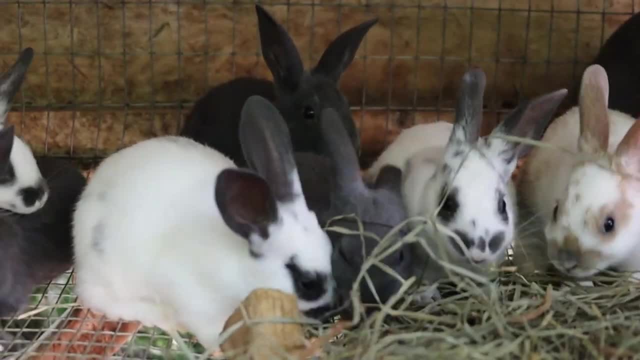 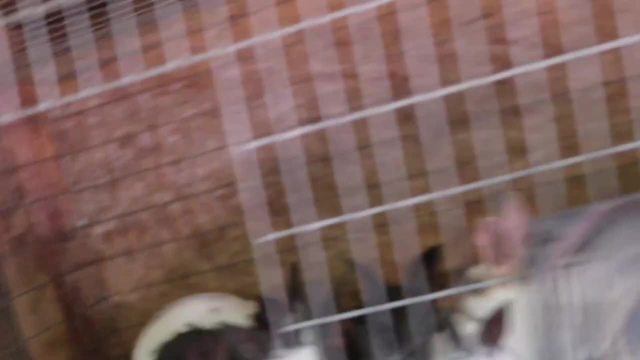 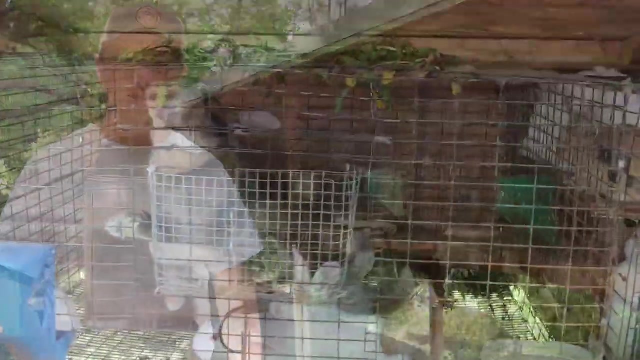 weaning your rabbits and you know putting them out on grass or into tractors, chicken coops runs, even extended systems. you know there's a lot of different ways that you can raise your rabbits and supplement your feed costs and you know you can feed your rabbits the things that you grow. you may. 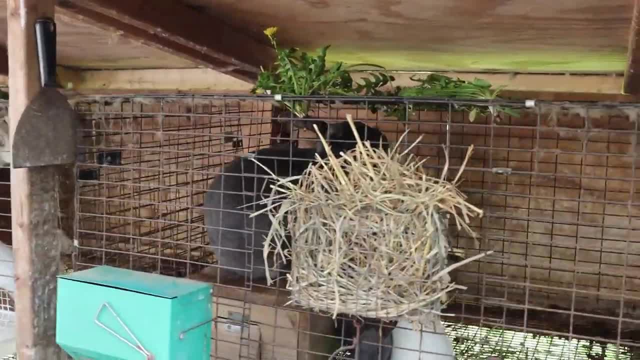 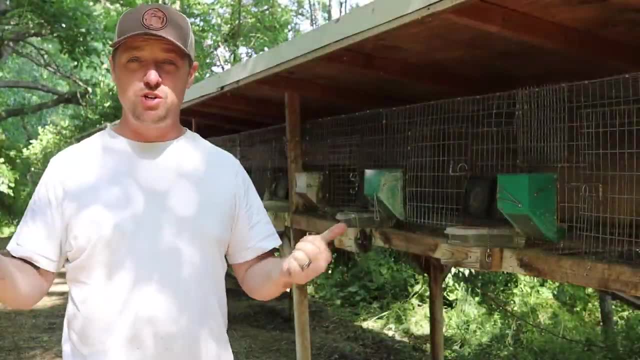 have losses if you're, you're introducing greens a little bit too early, when, if their stomachs aren't developed yet, you may have losses for other reasons. maybe you have some rabbits that are battling, some, some issues or some underlying issues you didn't know about when you got your rabbits, but in most cases 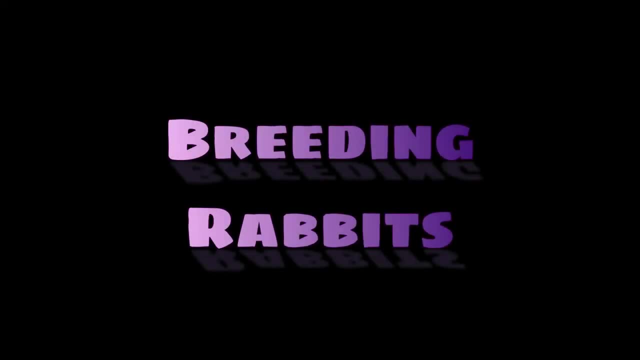 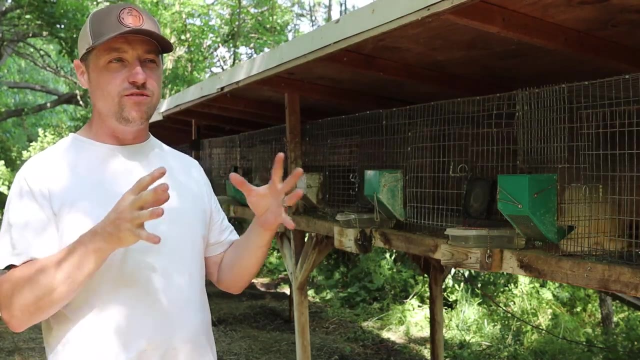 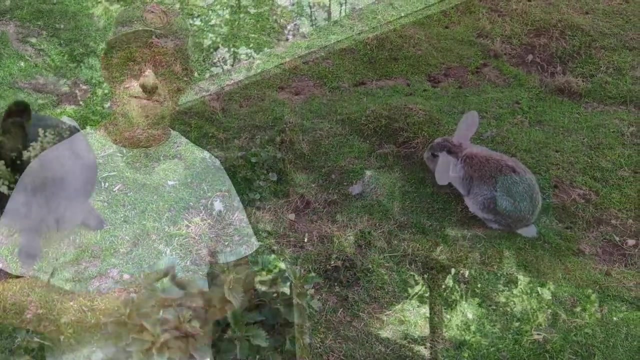 that's not why. so how many times have you heard breed like rabbits? you know, if you've been running a rabbitry, even for a short time. you know as well as I do that rabbits don't breed and have successful litters every time. so you know, just like other. 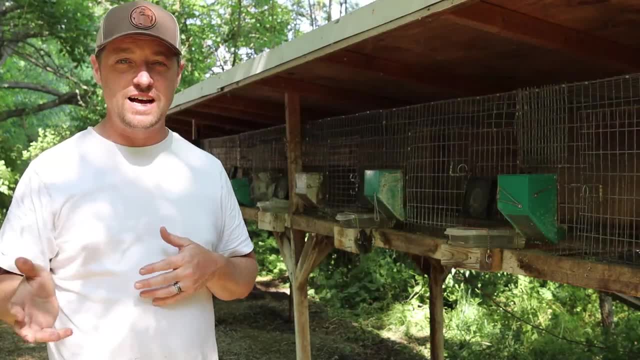 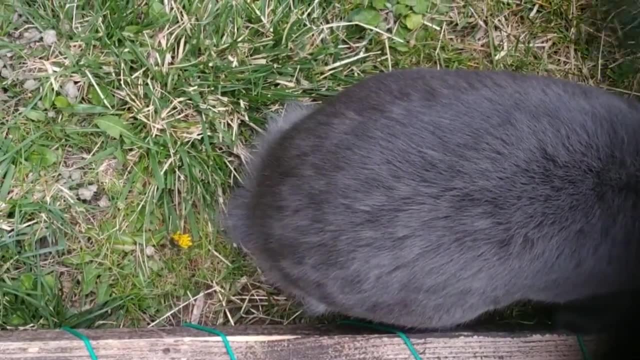 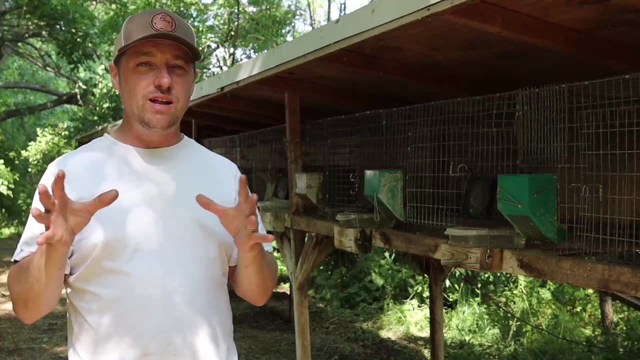 animals. they have hormones. there's estrogen, there's testosterone. you know she needs to mature sexually. he does. you need to make sure that that his parts are descended and her part is is swollen and there's a color change. you're looking for a red, swollen vent now. this will happen approximately around fourteen weeks a. 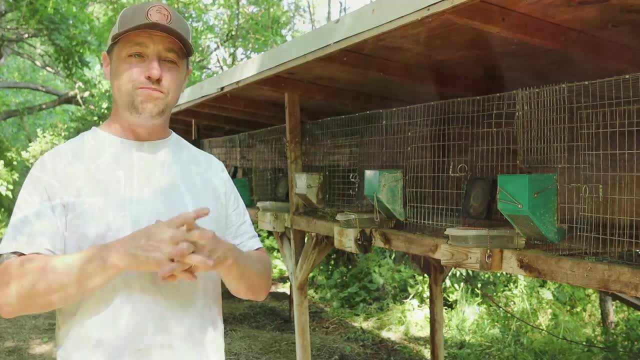 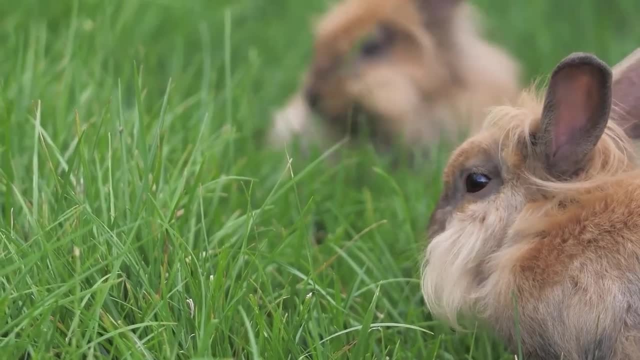 little bit sooner for the guys, a little bit later for the, the gals. but you know, folks often have luck because they'll breed, maybe they'll have a false litter, they'll rebreathe and they will have their litters. because you're gonna have success if you keep at it. but because there's things like table. 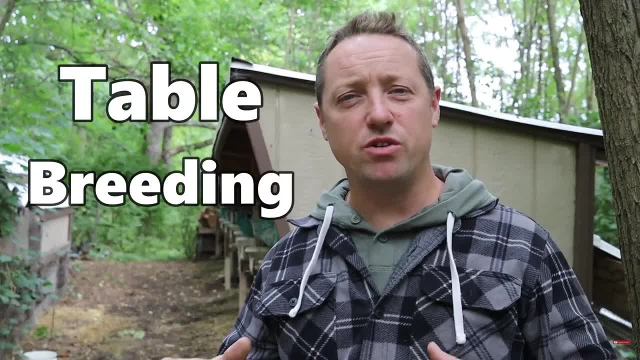 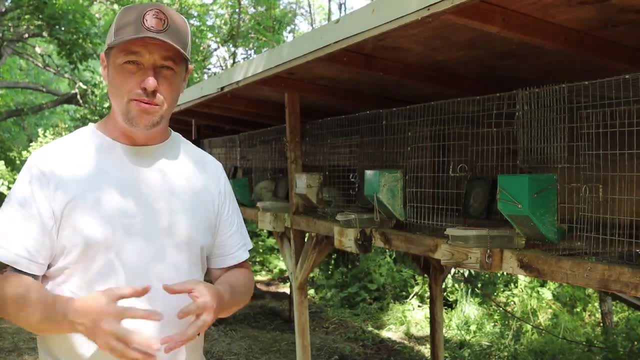 breeding where you can jumpstart your dough, and I can put a video up there if you like to see what that's all about. it's important that you understand. rabbits are induced ovulators, meaning that A rabbit just being near a buck or petting a rabbit 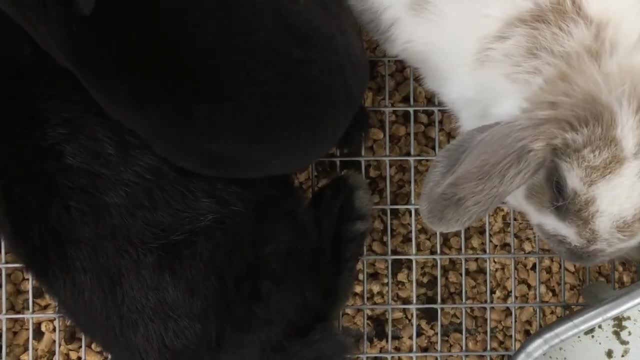 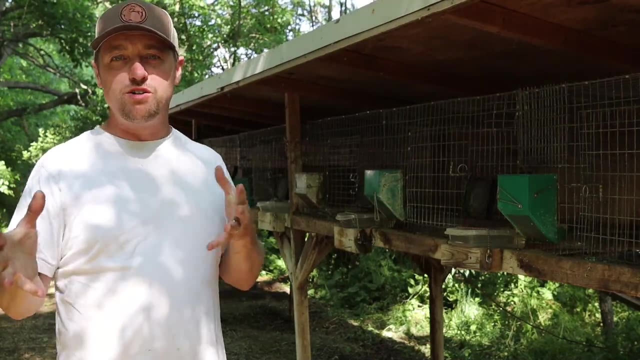 or a rabbit that gets mounted. even though it's not a fall off, she still may pull fur in two to three weeks because she's an induced ovulator. Her eggs will drop and it's important to re-breed, you know, eight to 10 hours. 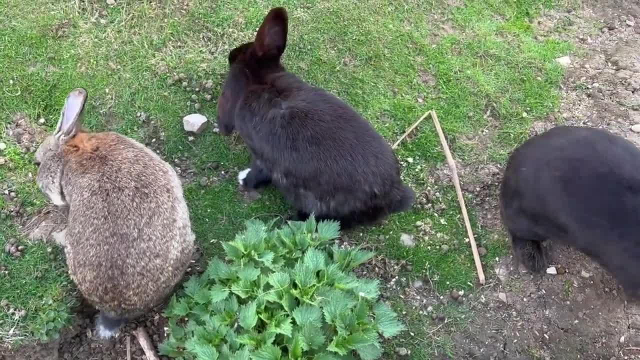 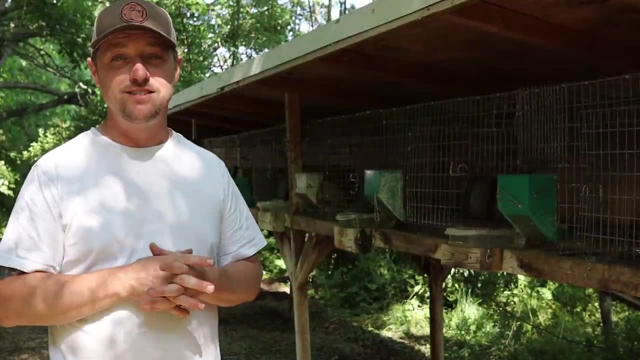 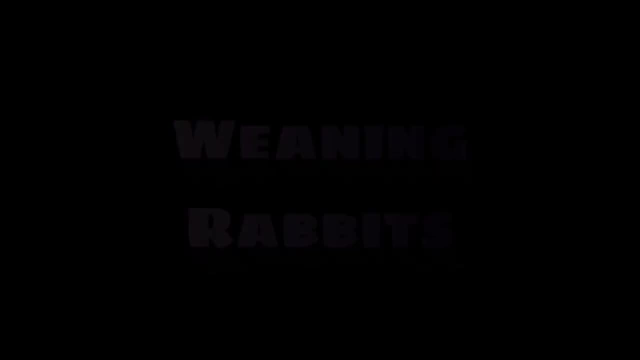 after the first time you bred her. This is a great time to make sure that you can fertilize the embryos, But that's actually not the number one reason most rabbit trees are failing. You know, when it comes to weaning rabbits, some folks think that they're weaning their rabbits too early. 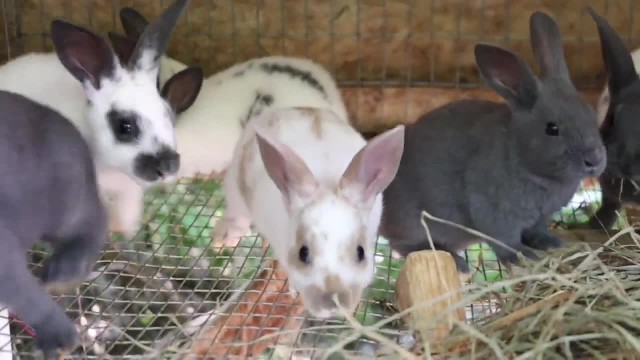 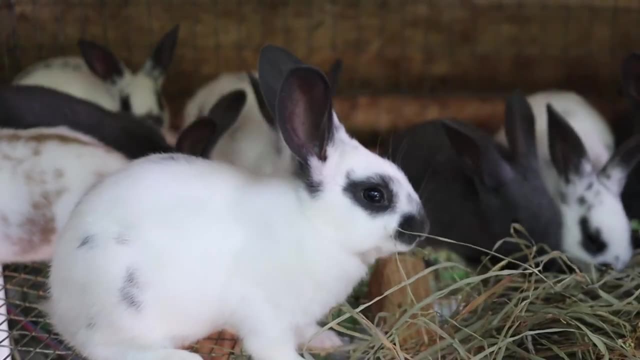 And if you're weaning them right around five weeks, six weeks, you know they've had enough time to get enough milk from mama to build a strong immune system. Now some folks want to leave their kits with their mama until nine- 10 weeks. that's too long. 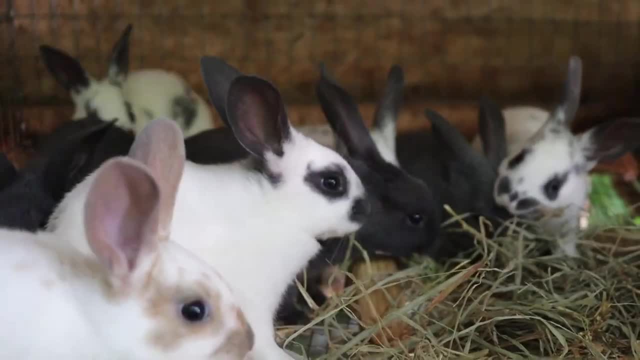 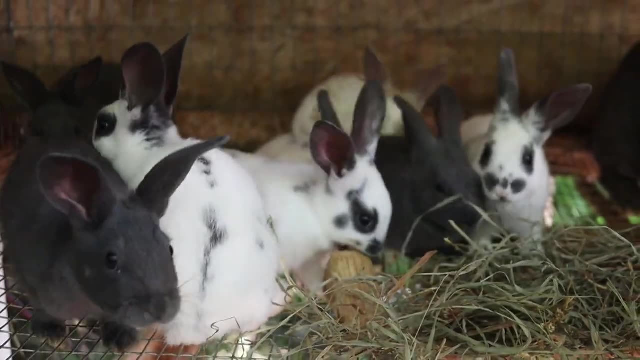 The factory is already dried up. They're already on to pellet and water. You know so. but understand that mama's milk is what you know. helps them build a strong immune system, helps them develop. helps them, you know. 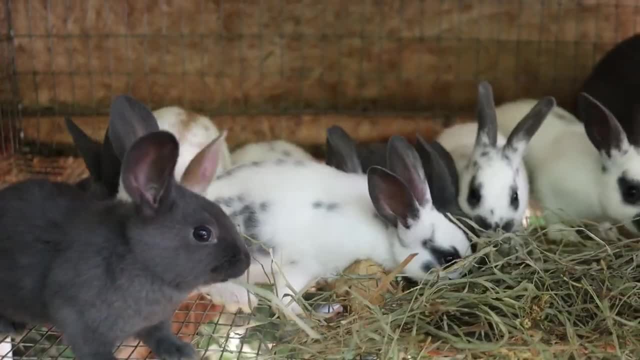 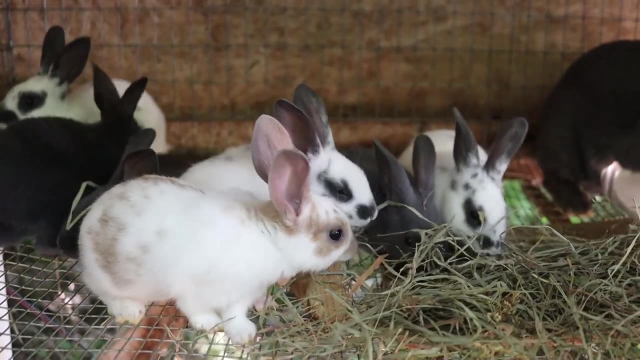 have the nutrition needed in order to be able to digest food and move forward. So you can wean really as early as four weeks, five weeks, six weeks. We usually shoot for about six, seven weeks, but that's not usually the number one reason. 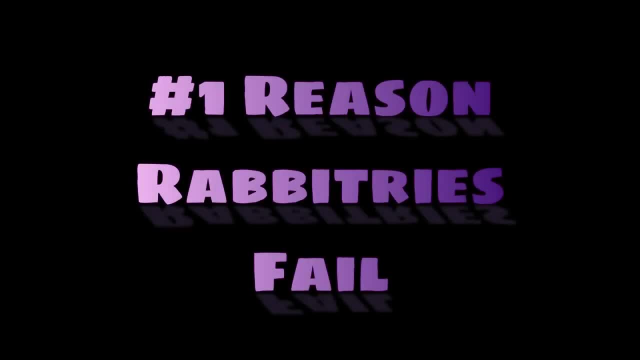 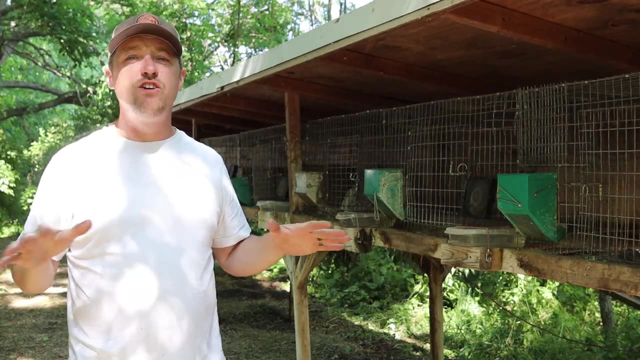 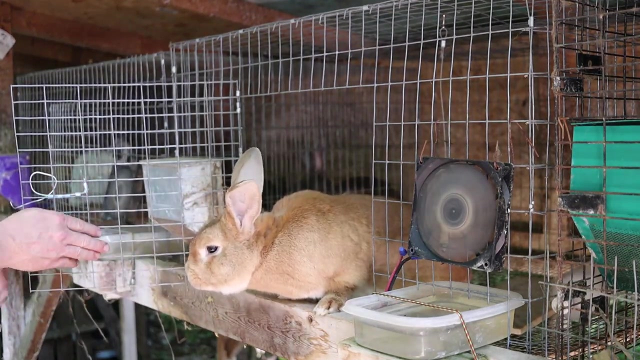 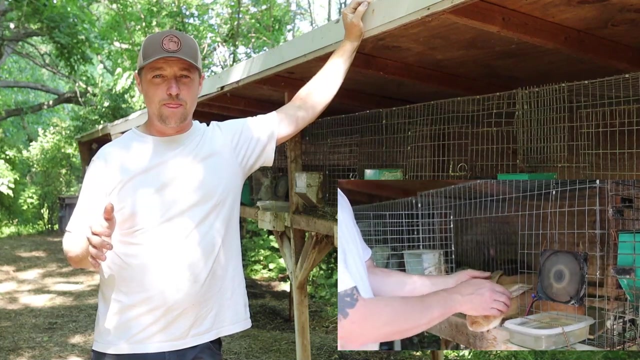 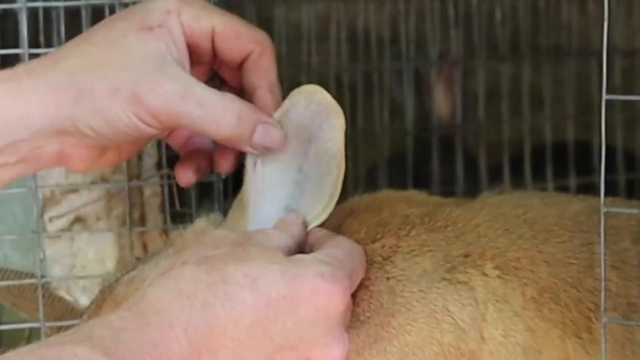 why folks are failing at their rabbitry. The difference between running your rabbitry blind or running your rabbitry with rabbit cards, rabbit data, copies of dates and breeders. keeping good records is the number one reason rabbitries succeed. I almost said that backwards. 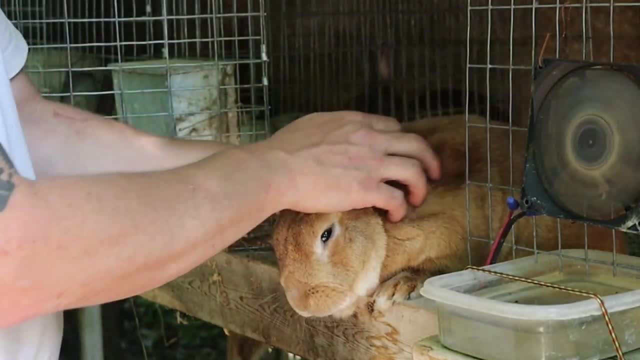 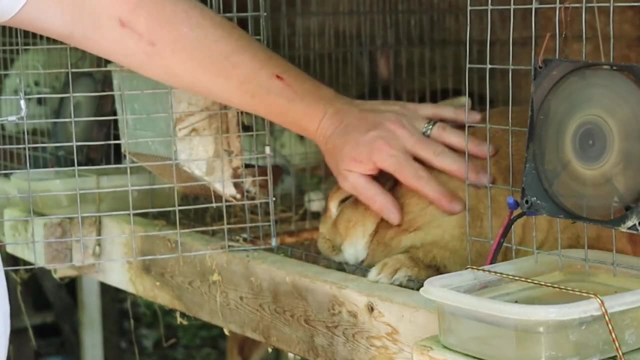 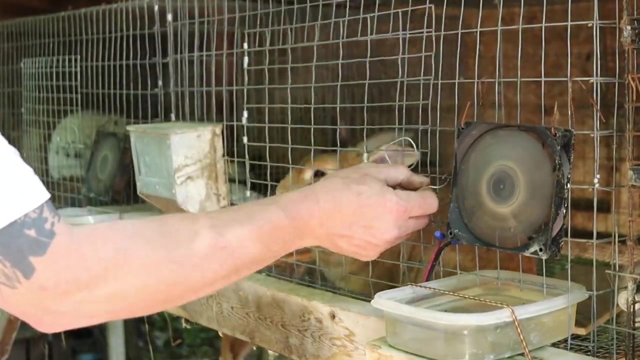 So in the past you've seen my videos- I always have cards up above the rabbitry. Okay, The rabbits now. I don't have them today, of course, but rabbit cards, pieces of paper, index cards, post-its of some sort with dates of birth, kindling dates. 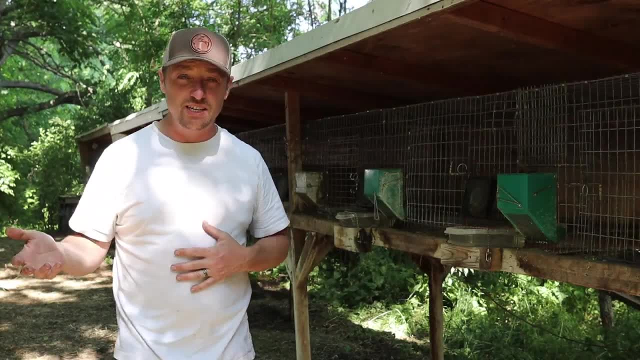 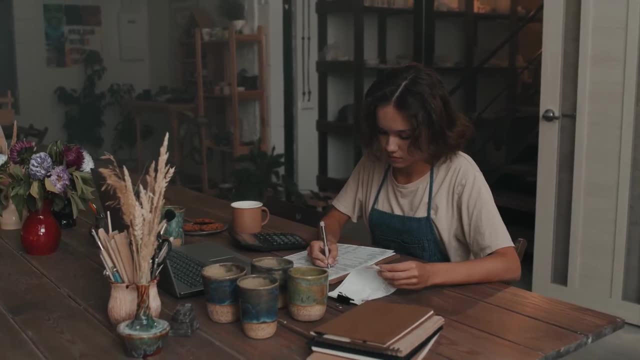 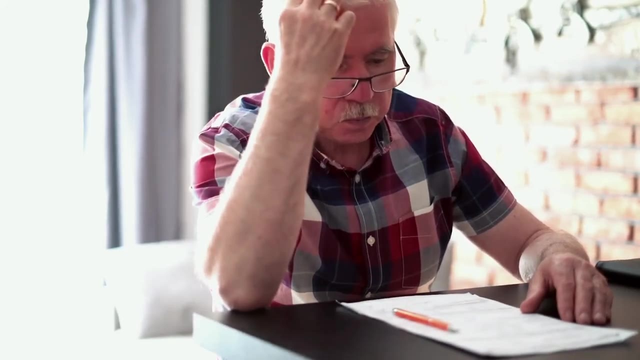 breeding dates, breeding partners, numbers of kits in the litter, rabbits that survived. All this stuff is important. Who bred with who when they bred. I got some good news for you, though. Some folks do not want to record all those dates. 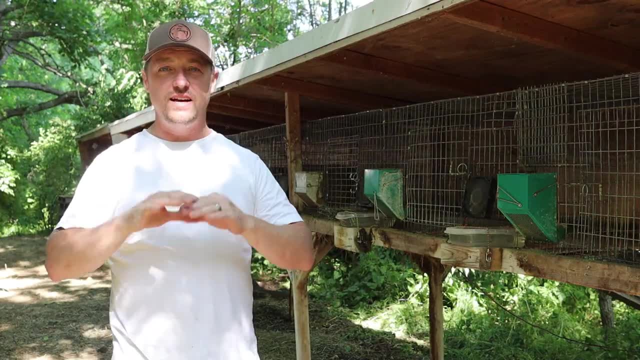 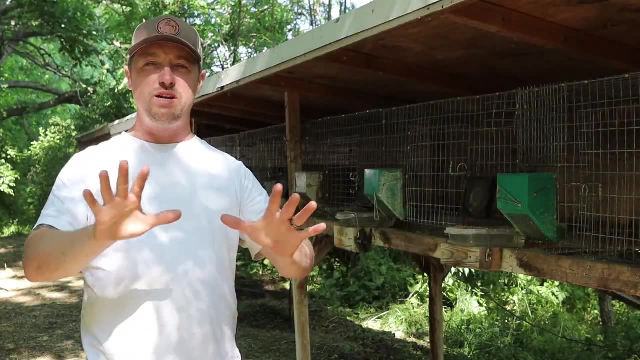 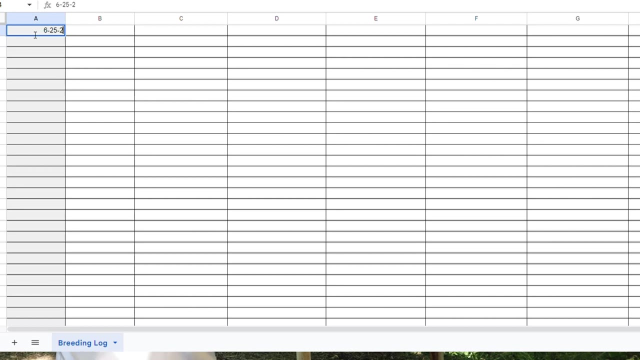 And we have made a kindling. we call it the kindling calendar because what happens is all the kindling dates. all you do is put in the day the rabbit was bred and it automatically produces your due date, your nesting box date, your removal date. 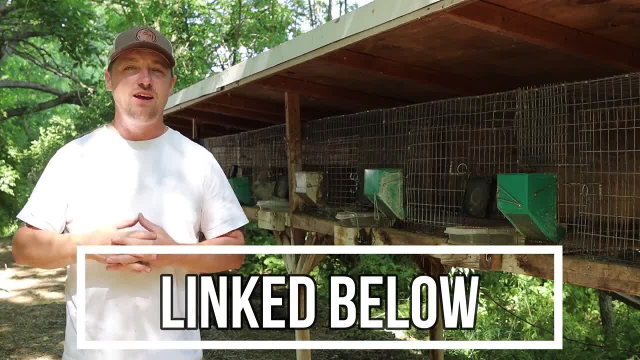 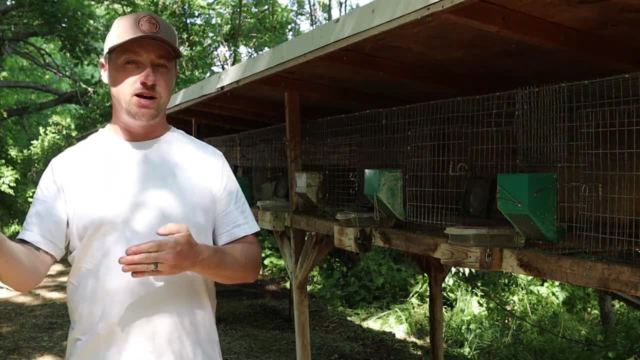 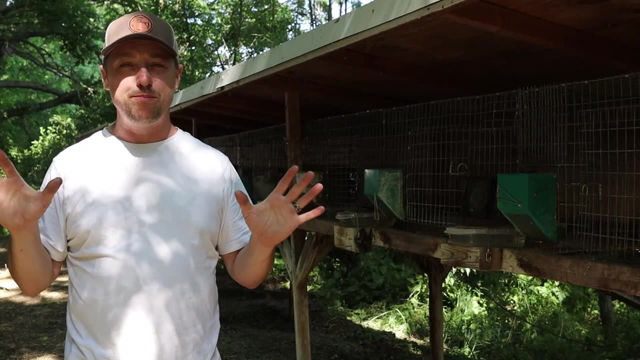 your rebreathe date, how many kits that litter had, And you always can put in the name the doe that was bred and the buck that she was bred to. But all you have to do is put the breeding date in and it's a one-time payment for $5. 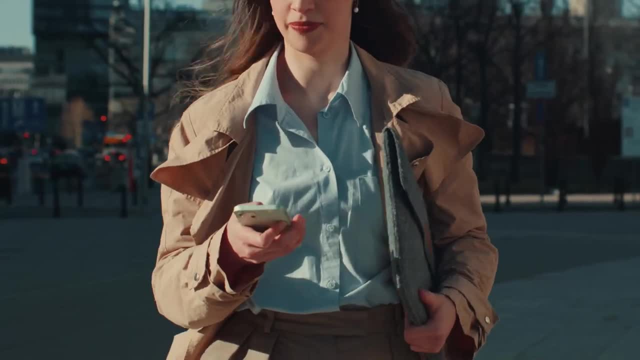 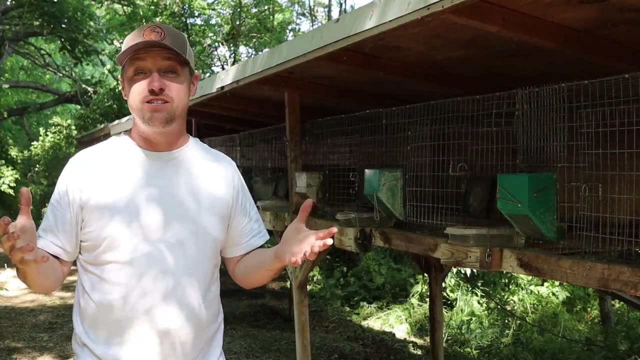 and you'll have it for life. It's an app that you can, that runs on Google Sheets, that you can have in your pocket in your cell phone. have it all the time. I'm really I'm excited about it And I've talked about it before, and I just really recommend it.